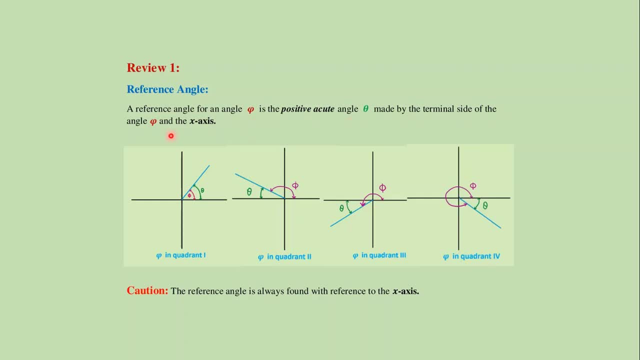 theta made by the terminal side of the angle, phi and the x-axis. So reference angle is always a positive, accurate angle and it also make with the x-axis. If an angle on the first quadrant, then this will be the reference angle. If an angle is on the second quadrant, then this: 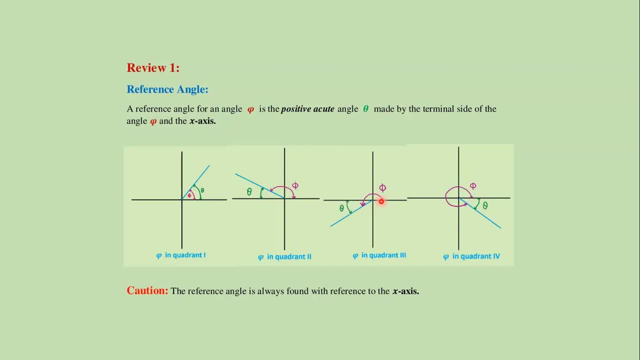 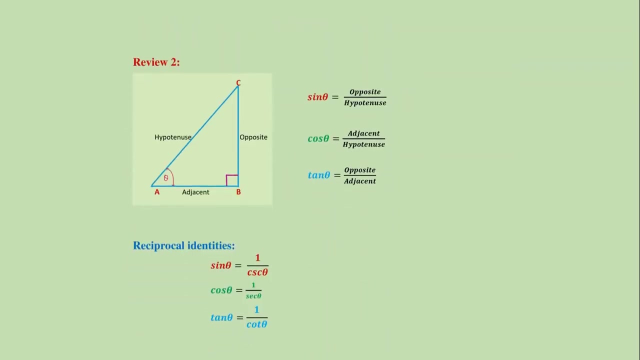 will be the reference angle. If an angle phi is on the third quadrant, then this will be the reference angle, And if an angle phi is on the fourth quadrant, then this will be the reference angle. We also need to review, like for any right angle triangle a, b, c. 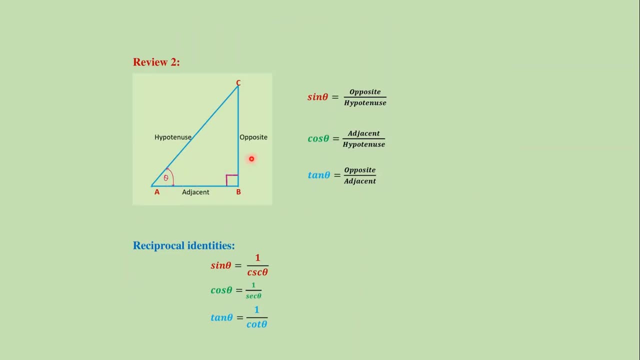 this angle is theta, then this will be the opposite and AB will be the adjacent and S is the hypotenuse. So sin theta is opposite over hypotenuse, cosine theta is adjacent over hypotenuse and tan theta is opposite over adjacent. We also need to review reciprocal 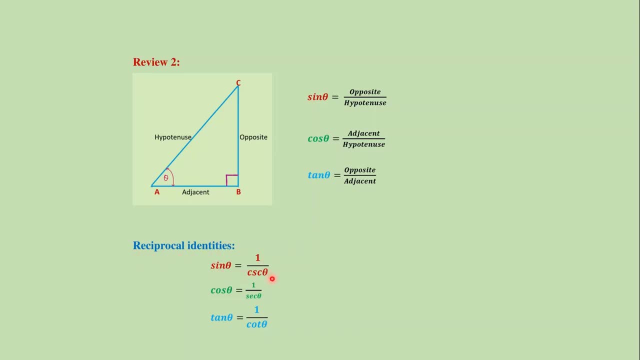 identities like sin theta is 1 over cosec theta, cosine theta is 1 over sec theta and tan theta is 1 over cot theta. Now we are ready for our main topics. Take a point P on quadrant 1, let us 3, 4.. So OQ will be 3 and QP will be 4.. And if you use Pythagorean, 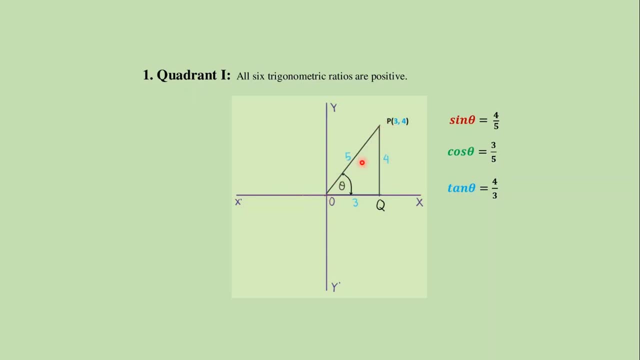 theorem, then you will get O equals to 5. And the reference angle will be this one and opposite is 4, this 3 is the adjacent and this 5 is the hypotenuse. So sine theta will be opposite over hypotenuse, that means 4 over 5, cosine theta will be: 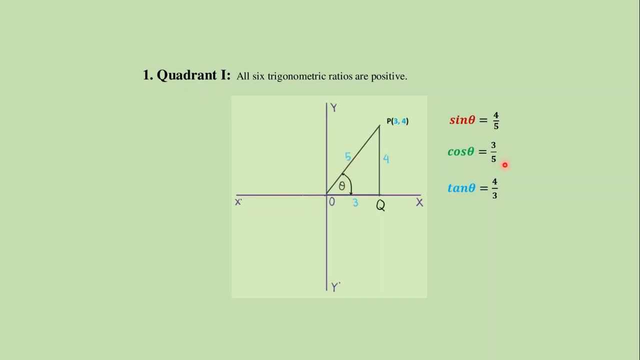 adjacent over hypotenuse. that means 3 over 5 and tan theta will be opposite over adjacent, which is 4 over 3.. Did you see? all of them are positive. Now go to second quadrant. So take a point P on second quadrant. that is negative 3, 4.. So this will be negative 3 and QP will be positive. 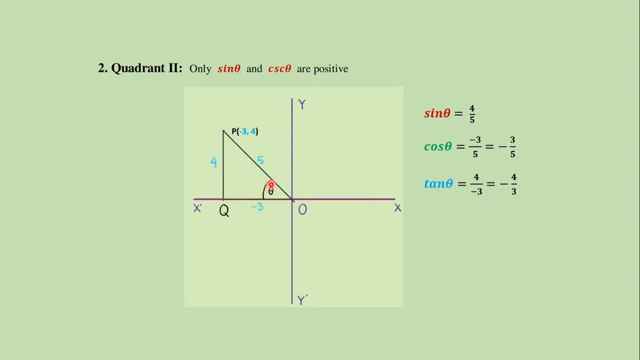 4 and the reference angle is this one. So this 4 is the opposite, negative, 3 is the adjacent and 5 is the hypotenuse. So sine theta will be opposite over hypotenuse. that means 4 over 3 and tan theta. 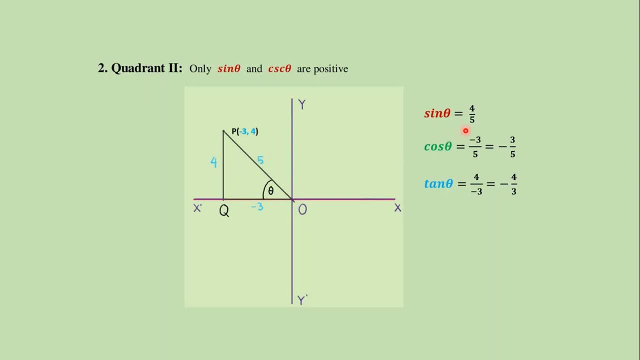 will be opposite over hypotenuse, which is 4 over 5.. Cosine theta will be adjacent over hypotenuse, which is negative, 3 over 5, negative 3 over 5, which is a negative number, And tan theta will be opposite over adjacent. that means 4 over negative 3, 4 over negative 3, which is a negative 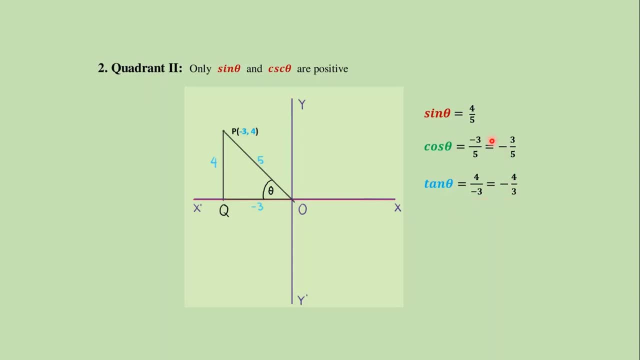 number. So did you see, on second quadrant only sine theta is positive and other two are negative, Since cosec theta is a reciprocal of sine theta, so cosec theta will also be positive. And on the third quadrant we know, only tan theta and cot theta are positive. So take a points. 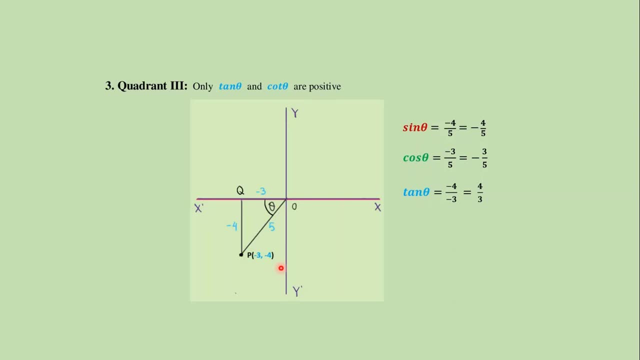 p, let its negative 3 negative 4.. So similarly you will get po equals to 5 and the reference angle will be this one. So opposite is negative 4, this negative 3 is the adjacent and 5 is the hypotenuse. So sine theta will be opposite over hypotenuse. 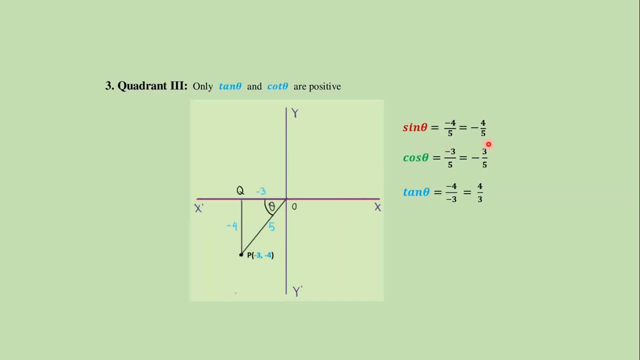 which is negative. 4 over 5, the negative number. Cosine theta will be adjacent over hypotenuse, that means negative, 3 over 5, negative 3 over 5, which is negative, 3 over 5, which is negative number. And tan theta will be opposite over adjacent, that means negative 4 over negative. 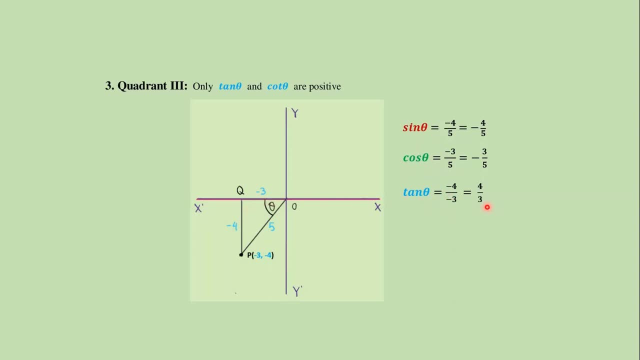 3, negative 4 over negative 3, which is a positive number. Did you see? on third quadrant, only tan theta is positive and other two are negative. Finally, take a point p on quadrant 4. let its 3 negative 4.. So, similarly, this distance is negative 4 and this distance is negative 4..